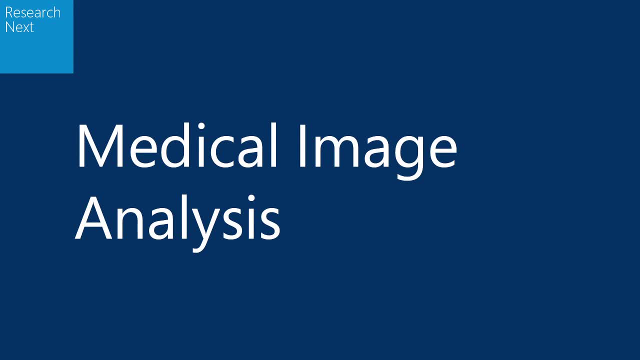 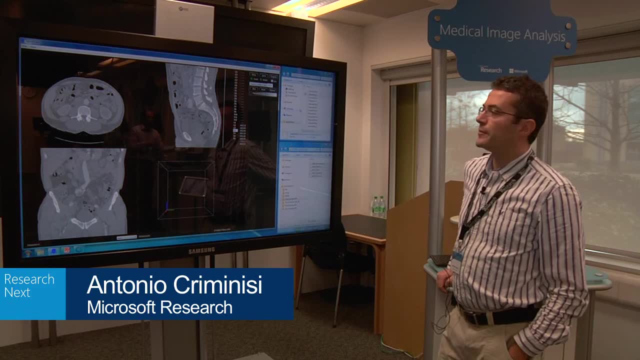 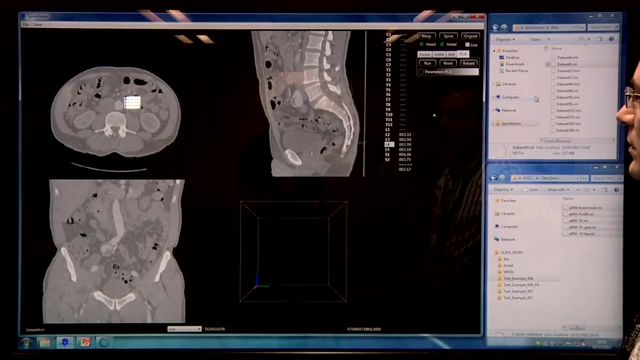 Hello, hi, good morning. My name is Antonio Criminisi and I work here at Microsoft Research in Cambridge, And the theme I'm going to be talking about today is about the analysis of medical images. In particular, it's about how to apply modern machine learning technique. 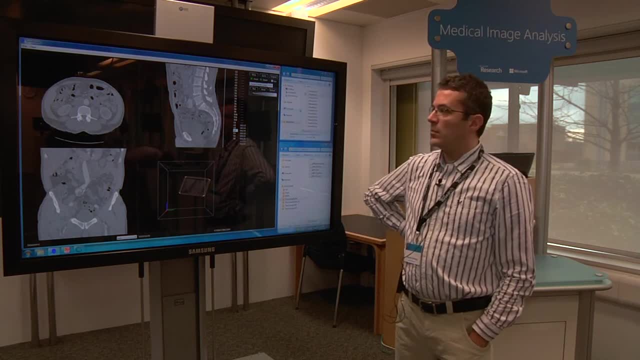 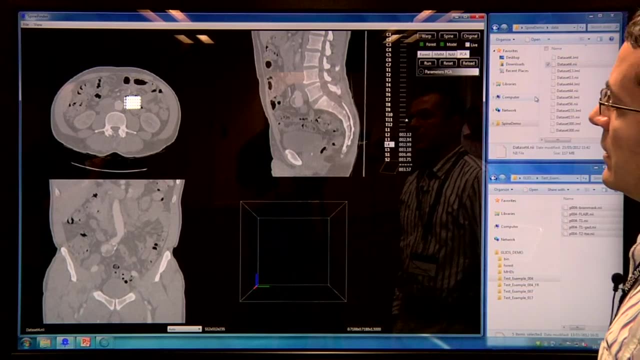 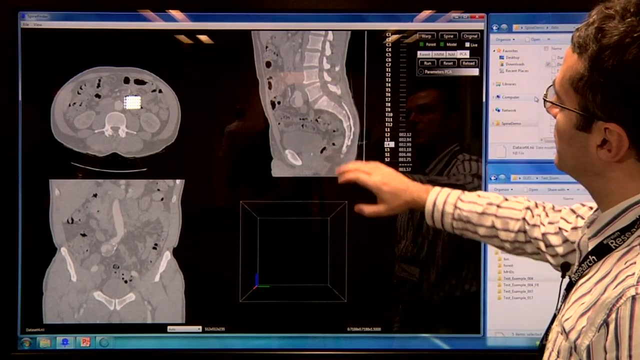 to the automatic analysis of medical scans. Medical scans are like this one that we're showing on the screen. This is a CT scan of a patient. CT stands for computed tomography, and you can. you know, even if you're not medically trained- you might not be- you can. 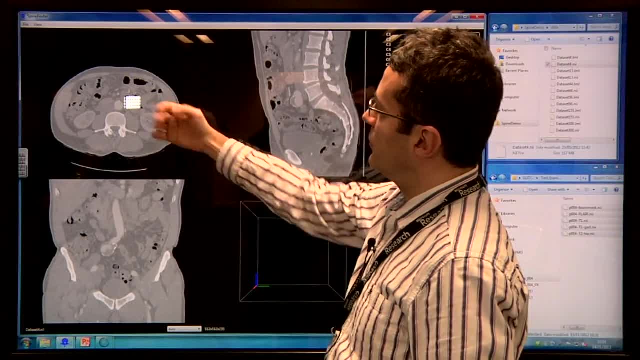 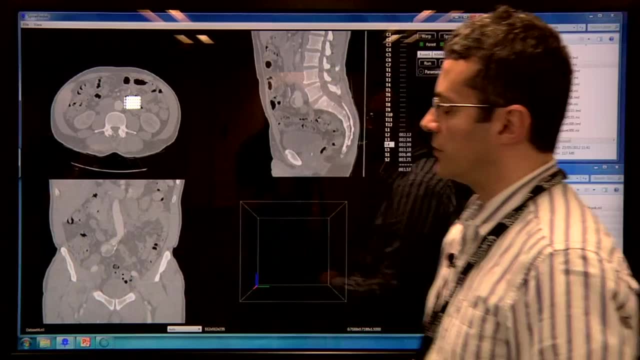 see structures like the spine. you know this is a view of the same patient. you know horizontal view, and this is a frontal view, And you can see the pelvic region and the aorta. Now, what we're trying to do here is we're trying to come up with tools that can help the 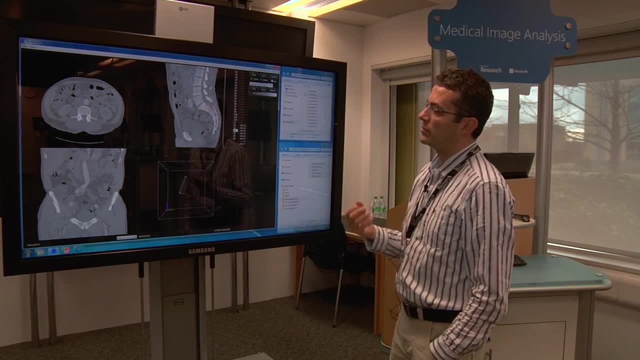 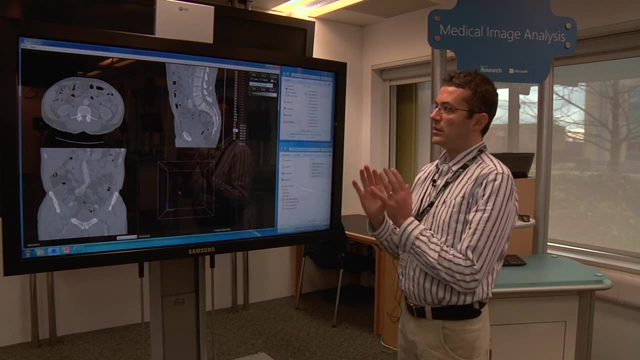 doctors, you know, diagnose a problem, you know with a patient and also treat, you know, the problem more efficiently. In particular, what we're trying to do, you know, we're trying to make you know the analysis of medical images quantitative so that you can really 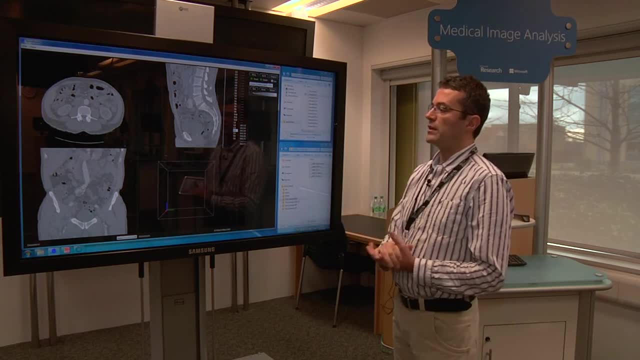 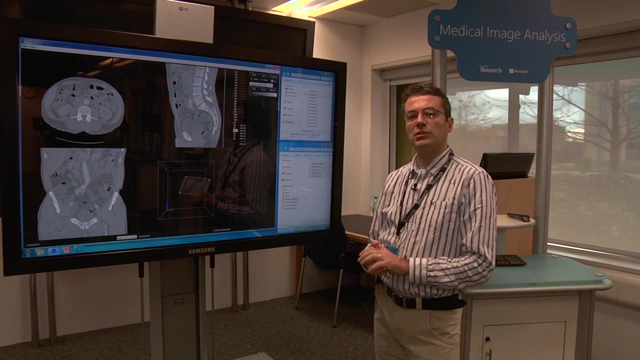 assess how big, say, a tumour is, you know how effective a certain drug is. So we have two demos, one to do with the analysis of, you know, CT scans and the other one to do with the analysis of magnetic resonance scans of a patient's brain. 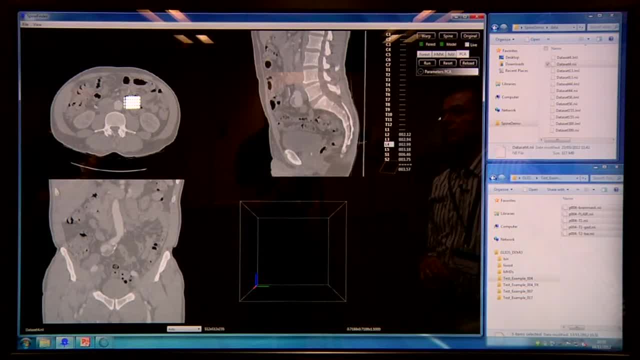 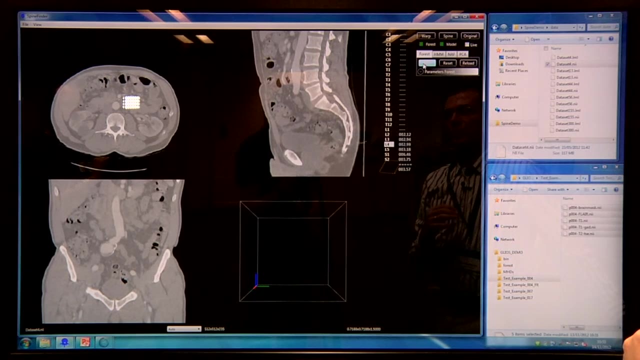 In this demo we have already loaded, you know, a patient image Again. you can see the different, you know, horizontal views here and the different side views of the patient here. What we do is, first of all, we want to automatically identify, you know, the spine. 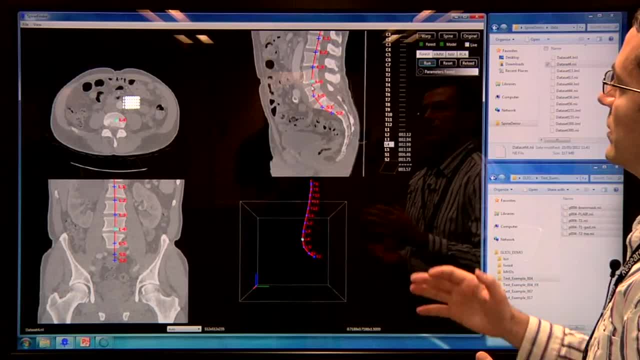 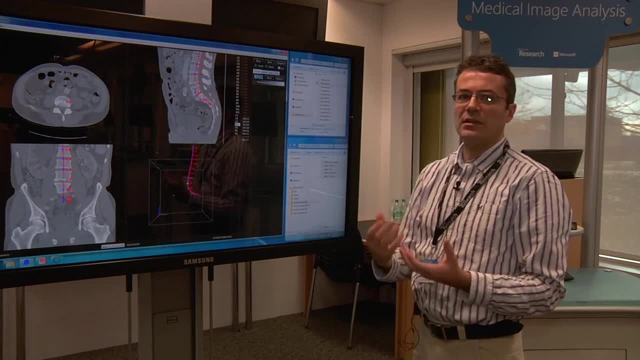 So the spine, you know, is important to identify, not just, you know, to be able to analyse whether there are broken vertebrae, But also because the spine is a natural coordinate system for the patient. So it is a very helpful. 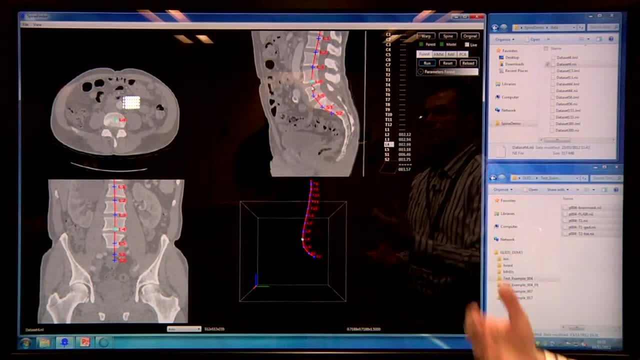 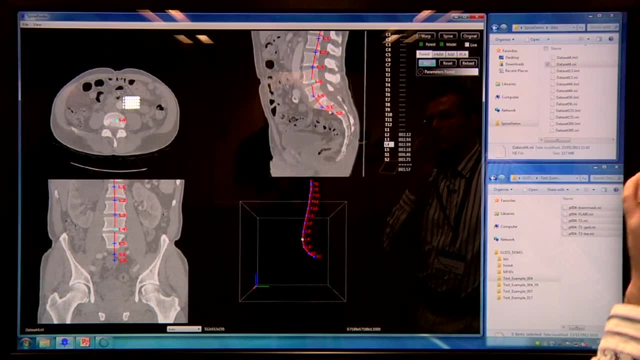 thing to do for any kind of doctor that you know wants to look at these sort of images. So you have seen that. you know I've clicked on the run button and something has already happened very, very quickly. But it is not, you know, quite, as you know, refined as it. 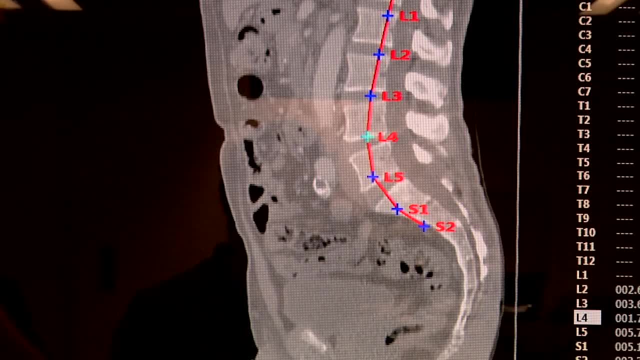 could be. So then I launch a second round of refinement and you can see the position of the spine and the individual vertebrae. You know being refined, you're on the go. So now it's done After a few seconds. you. 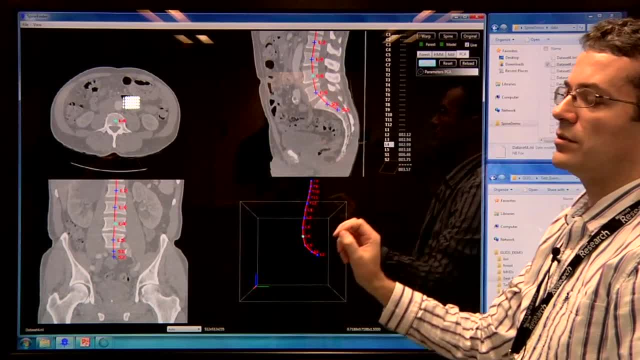 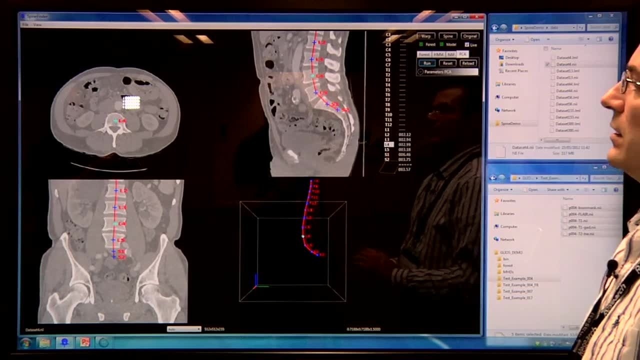 already have a very good idea of where the spine is, And not only that, you have the exact name for each of the vertebrae. So you might think that this is something that any trained radiologist would be able to do very, very quickly. It turns out that it is a little bit, you know, time consuming. 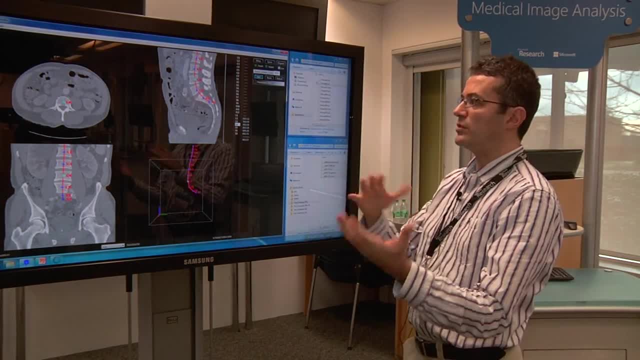 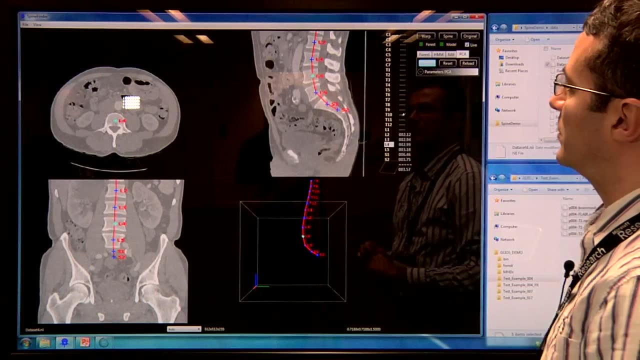 for them, too, to be able to do these sort of things, And they have to change between different views. So you can see that the vertebrae are looking at something you know from. you know the head towards the bottom to figure out which vertebrae they're looking at. 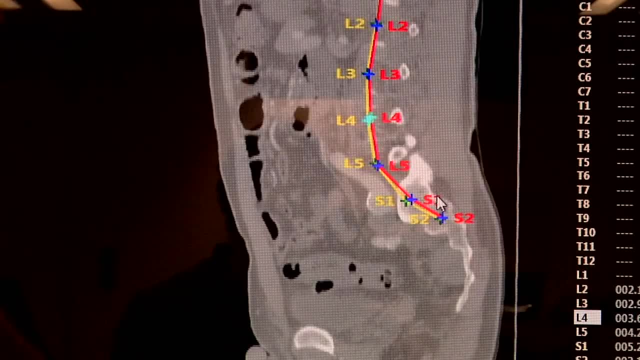 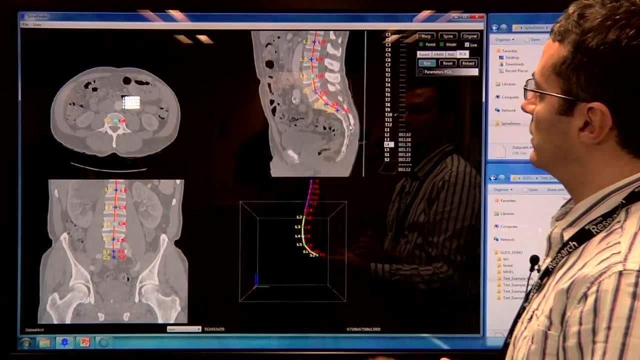 So we can also compare and really quantitatively measure how well we do with respect to some ground truth labeling. And so now you can see in red the automatically detected vertebrae and in yellow the ground truth position, And you can see that there is very good, you know. 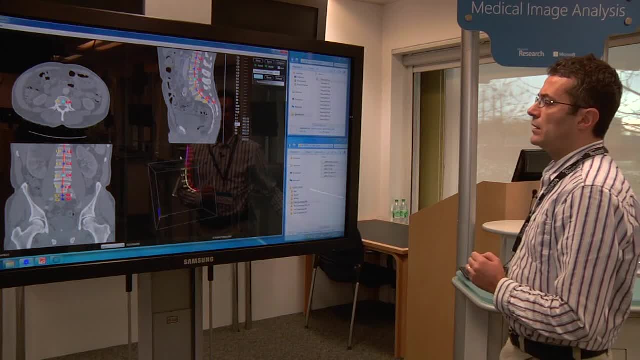 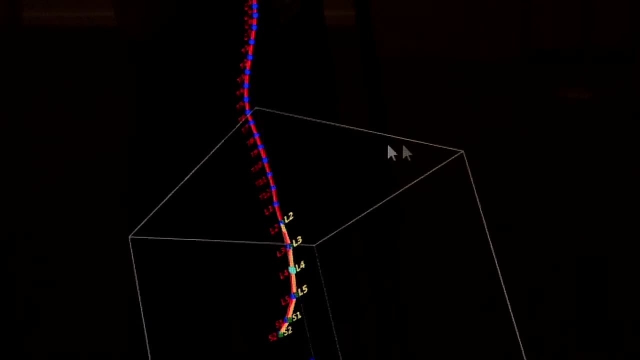 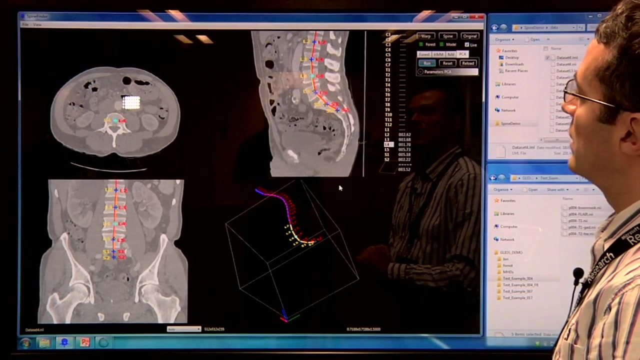 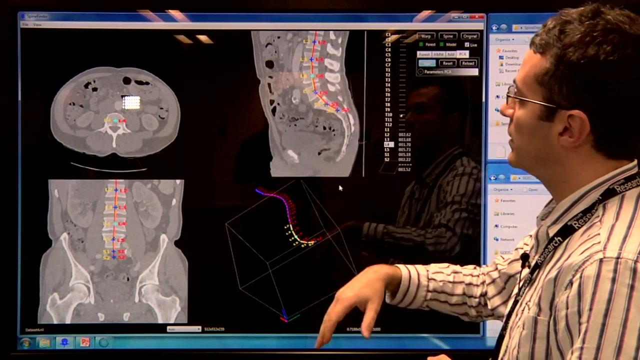 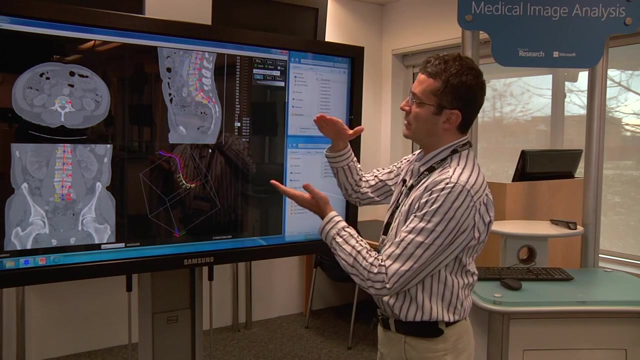 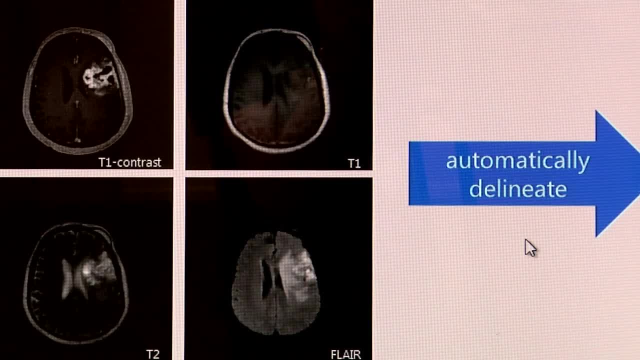 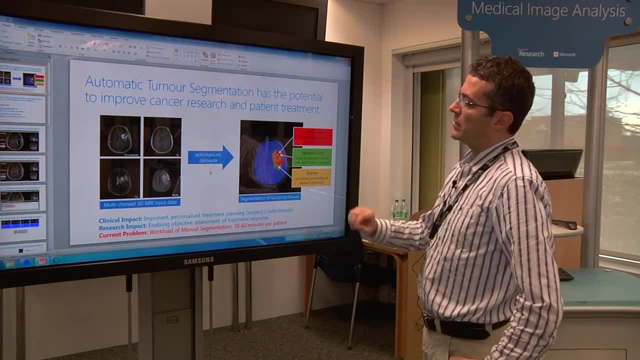 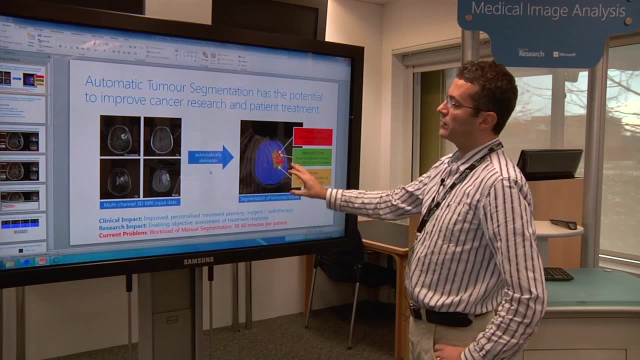 develop an automatic analysis tool which can tell us not only that this patient has got glioblastoma and how big it is, but also we want to figure out what are the different component regions in the tumor. This is color coded here in this view: where? 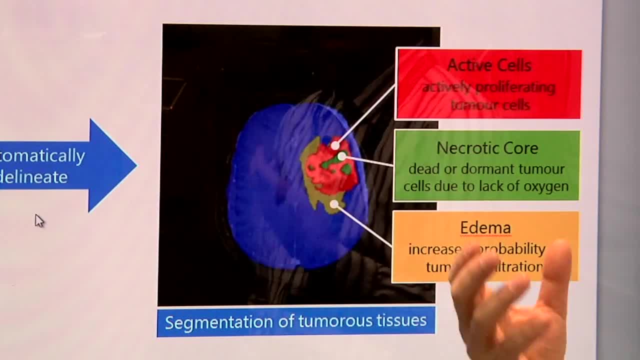 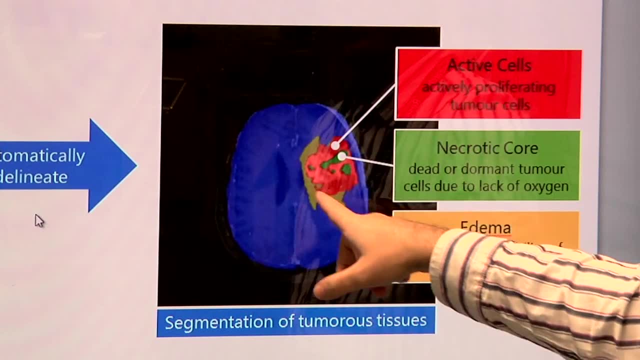 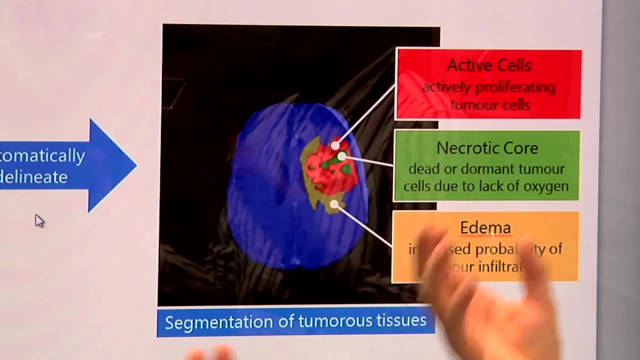 blue means healthy tissue and then green means necrotic core, which is the already damaged, in fact dead, region of the brain. Red is the actively proliferating region where there is a lot of oxygen blood being drawn into the area because the tumor is feeding itself and growing very rapidly. 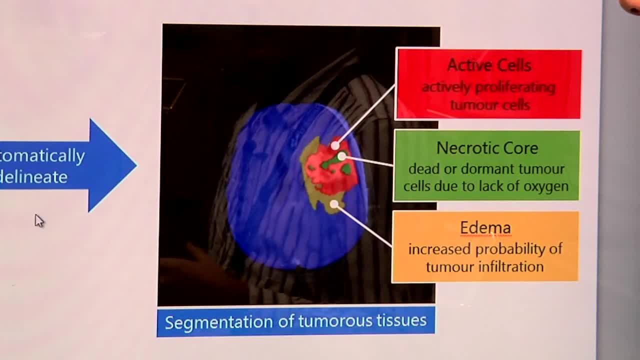 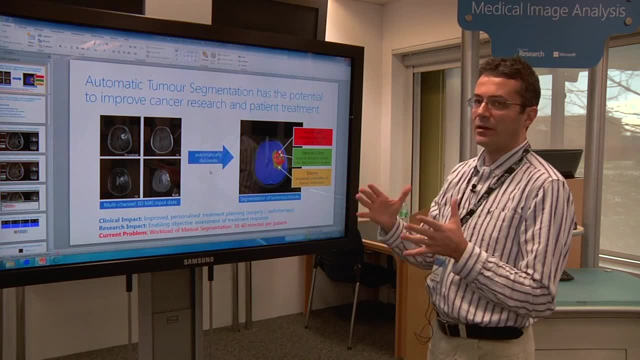 and yellow is what's called the edema, the inflammation, where it might be possible that you find tumor cells in there as well, but in general it's just a healthy inflamed region, but it's something to watch very carefully. So what do we have here? 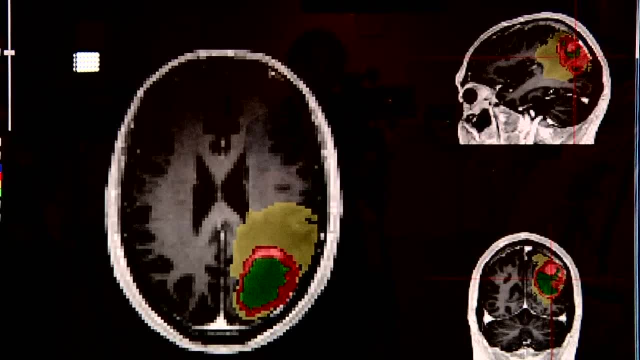 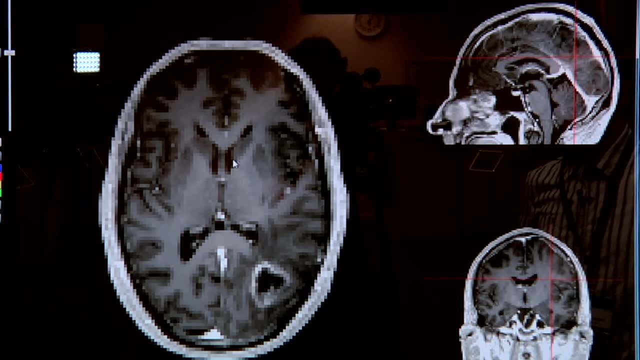 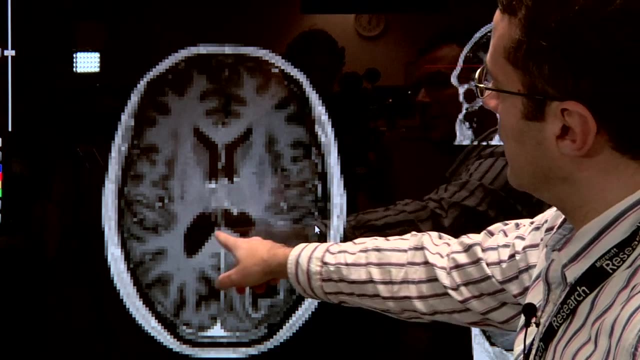 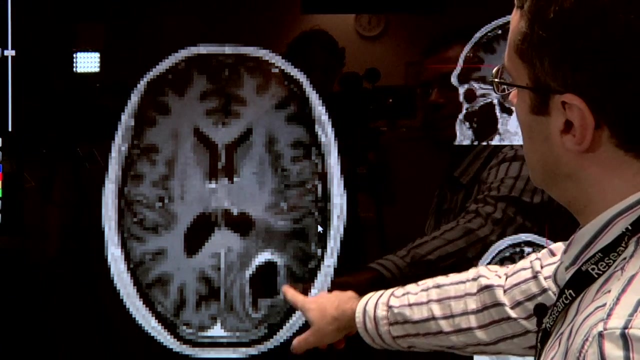 We have another application. I'm just going to select a patient, drag the images there, the images get loaded and here you have the tumor. So what you see here, these black regions, this is all healthy. they're called ventricles. all this region here is all healthy. but this region here where you see this,